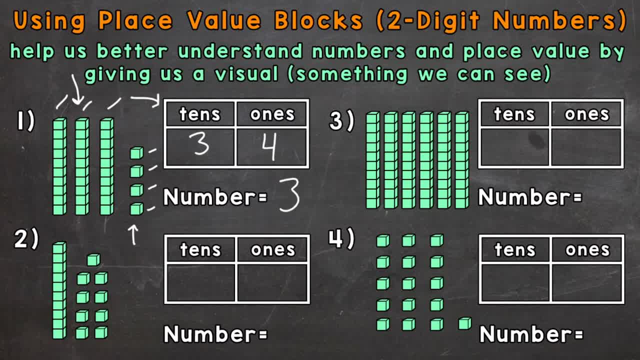 So, standard form, we have 34.. And to recap here, this four represents four ones, four individual blocks. The three represents three groups of 10, which has a value of 30. And that gives us the number 34.. On to number two. let's count our ones. So we have one, two, three, four and five. 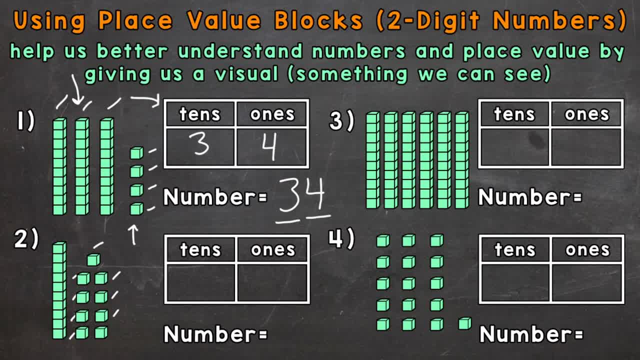 Six, seven, eight, nine ones there, So let's put a nine in the ones place to represent that, As far as tens go, we have one stack of 10, which has a value of 10. So let's put a one. 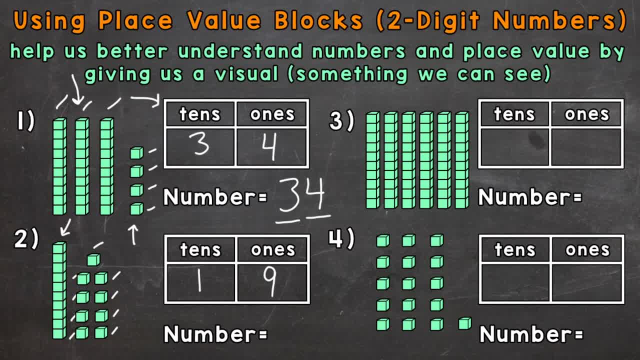 in the tens place to represent that one group of tens which has a value of 10.. Standard form: we have 19., 19. Nine representing nine ones, And then one representing one group of 10, which has a value of 10.. 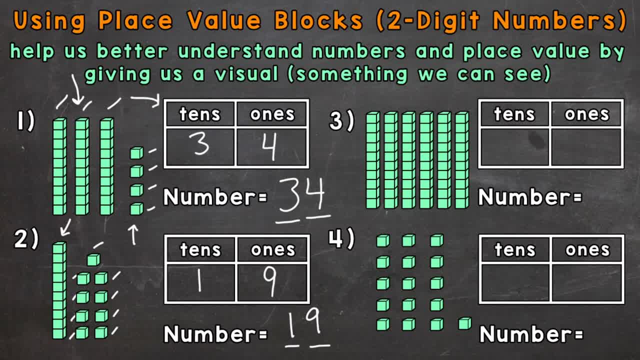 Number three: we'll start with the ones, but we don't have any ones, which is OK, that happens. So we represent that by putting a zero in the ones place. Now let's see how many tens we have: One, two, three, four, five, six groups of 10,. 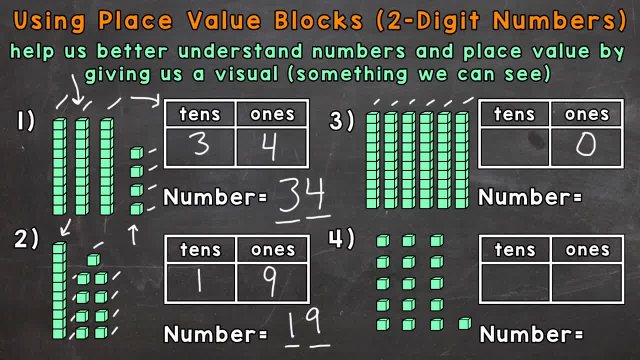 which has a value of 60. So we will put a six in the tens place to represent that. So our number in standard form is going to be 60. So we will see there how important that zero is in the ones place, because without it- let's look up here above our place value- 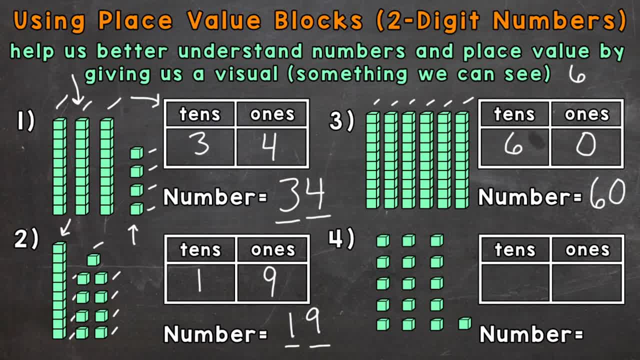 table, we would just have a six. That's a lot different than 60. We needed that zero in order to represent zero ones, and then the six in the tens place, which represents 60. So don't just put six for that one. Make sure we have zero in the ones place. 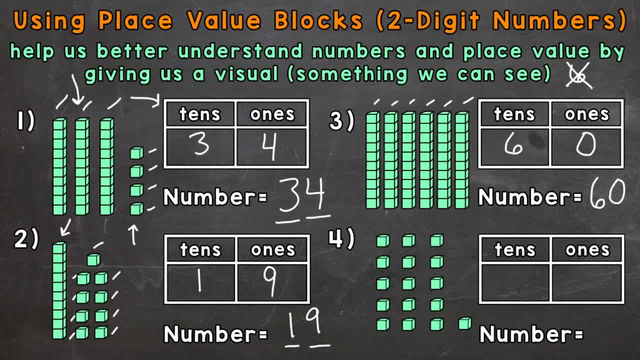 Lastly, number four, let's count our ones. So we have one, two, three, four, five, six, seven, eight, nine and ten. So we actually have a group of 10 there. So we can group that. It was not put into a stack.